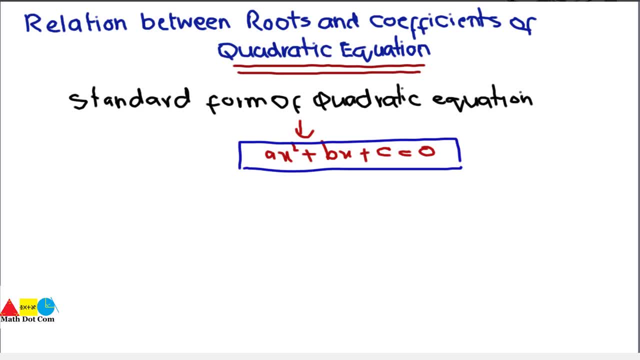 Roots are basically the values of x that satisfy the given equation. So the roots of the given equation can be found by By using the quadratic formula. But now this is not our concern. Currently we just know what are the roots of the standard form of quadratic equation. 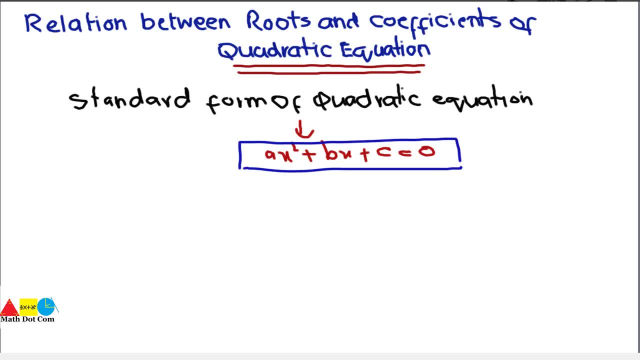 We have already seen in our previous lectures that how to find the roots by using the quadratic formula of the quadratic equation. So currently I will just write the roots of this quadratic equation. So its roots are b plus under root b, square minus 4ac divided by 2a. 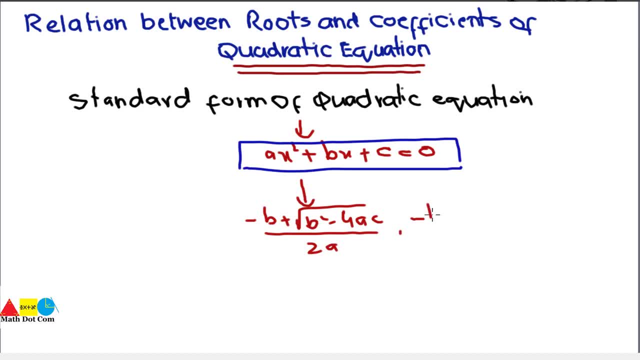 This is one root and another root is minus b, minus under root b, square minus 4ac divided by 2a. So these are basically the two roots of the standard form of the quadratic equation And how you can find How you can find these two roots. 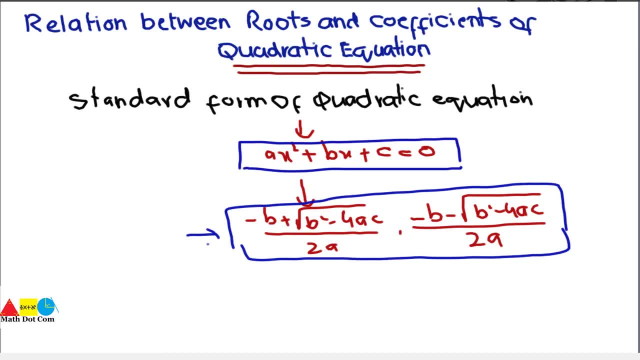 These two roots can be found by using the quadratic formula. Okay, After this, our concern is with the coefficients of the quadratic equation. Now, what are the coefficients of the quadratic equation? Let's write them: a, b and c. Okay, 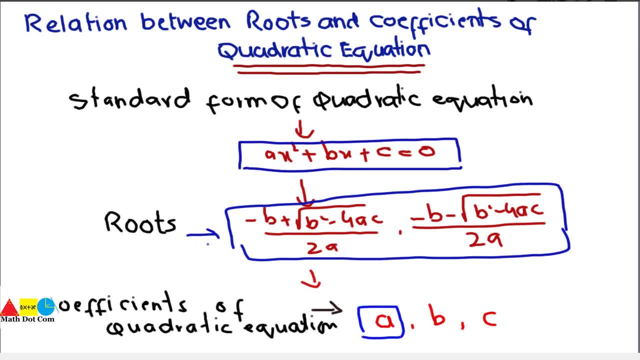 Where this a is the coefficient of x square, This b is the coefficient of x And this c is the constant term in the standard form of quadratic equation, as it is clearly seen from here, that a is the coefficient of x square, b is the coefficient of x and c is constant term. 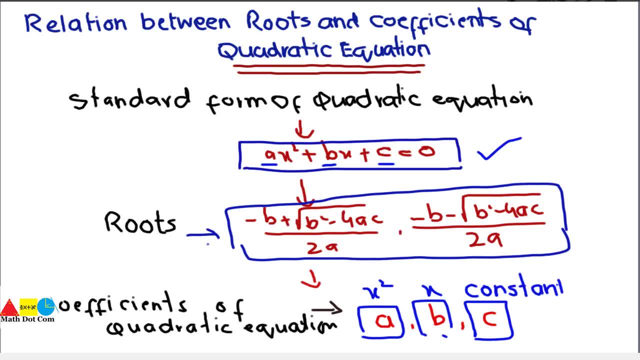 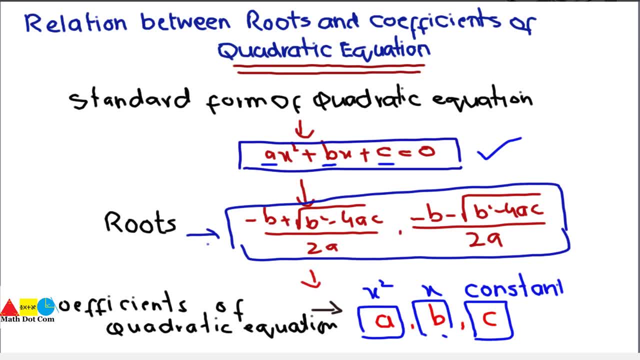 So what we actually required in order to find the relation between the roots and coefficients of the quadratic equation, So what we actually required in order to find the relation, are roots and coefficients of the quadratic equation. So by using these roots, we can find the relation between the two. 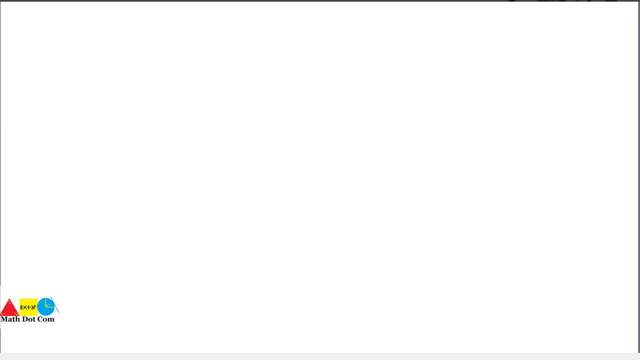 So let's find the relation between the roots and the quadratic equation. So, in order to find the relation, what we can do, we can say that let's say alpha, let's say that alpha is equals to minus b plus under root b, square minus 4ac divided by 2a. 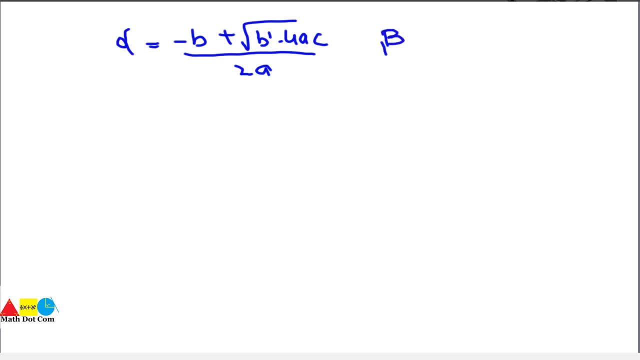 And beta is equals to, and beta is equals to minus b, minus Under root b, square minus 4ac divided by 2a. But we have done in this step. In this step we have assumed that let alpha and beta be the two roots of the quadratic equation. 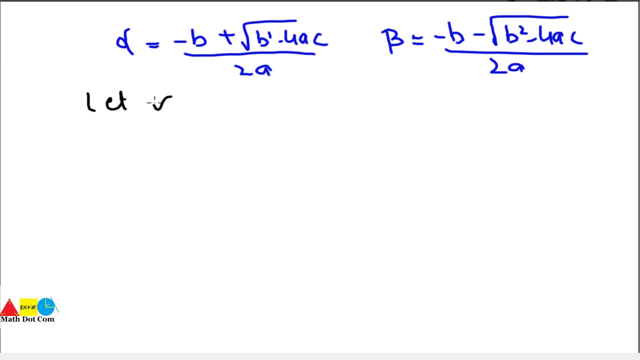 So I can write that let alpha and beta be the two roots of quadratic equation. So instead of writing these two roots in completely because of their complex form, we can replace them with alpha and beta. ok, now we have to find the relation between what we have to. 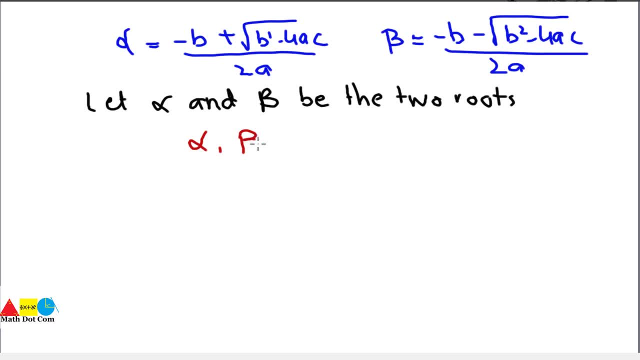 find the relation between alpha, beta, a, b and c. why? because alpha and beta are the roots of quadratic equation and a, b, c are the coefficients and we have already seen in the start of the lecture that we are going to find the relation between them. so, in order to find the relation, 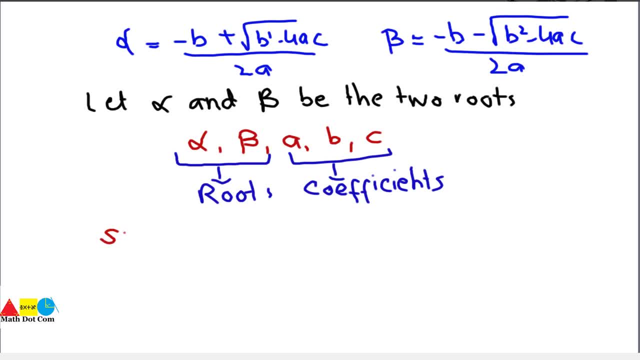 let's say that sum of roots of quadratic equation is equals to alpha plus beta. ok, so we can find: first we will find the sum of roots, then the product of roots and from here we will find the relation between them. so we will put the value of alpha and beta here in order. 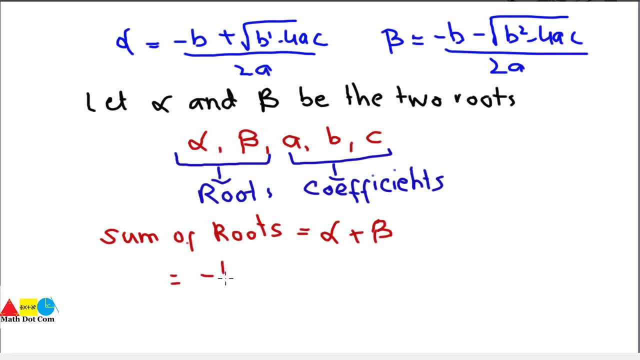 to find the relation as: the alpha is minus b plus under root b, square minus 4 a- c, divided by 2 a. plus beta is minus b minus under root b square minus 4 a- c, divided by 2 a. now we will take the LCM as minus b plus under root b square minus 4 a- c, divided by 2 a. now we 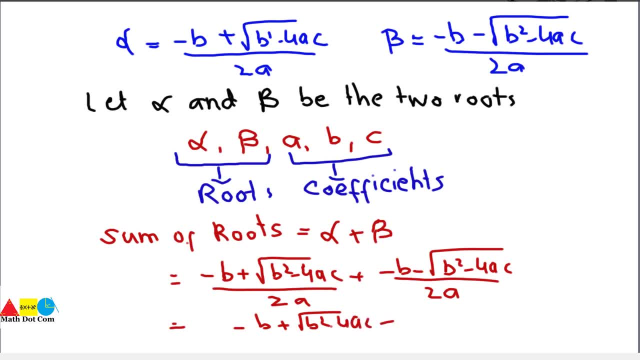 will take the LCM as minus b plus under root b, square minus 4 b plus under root b square minus 4 a c divided by 2 a. so it will be cancelled out. but we will get minus 2 b divided by 2 a. it will be cancelled out, and we will get minus b over a. so sum of roots is equals to. 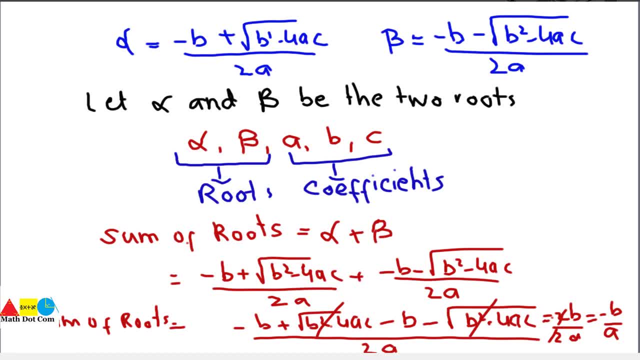 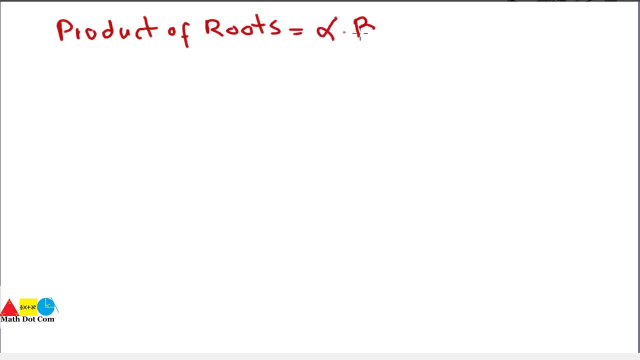 minus b over a. ok, now we will find the product of roots. So product of roots will be equal to alpha, dot, beta. We will put the value of alpha and beta. Alpha is minus b plus under root b square minus 4ac divided by 2a, and beta is minus b minus under. 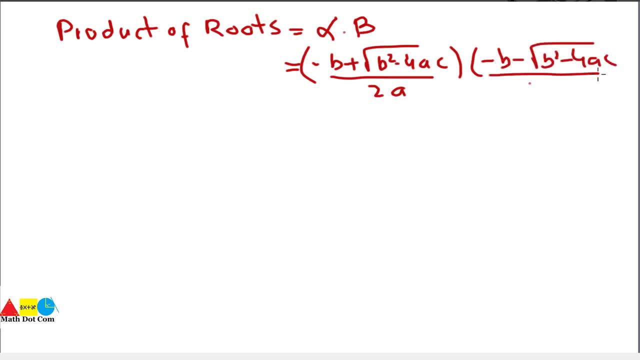 root b square minus 4ac, divided by 2a. We will multiply them together as b square plus b under root b square minus 4ac minus b under root b square minus 4ac minus under root b square minus 4ac, whole square divided by 4a square. So it will be cancelled out. We will get b square. 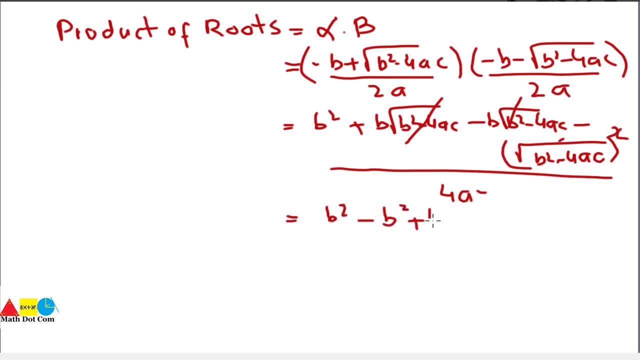 minus b square plus 4ac divided by 4a square. So it will be cancelled out, Hence 4ac divided by 4a square. cancelling 4 and 4 and a with the square, we will get c by a. 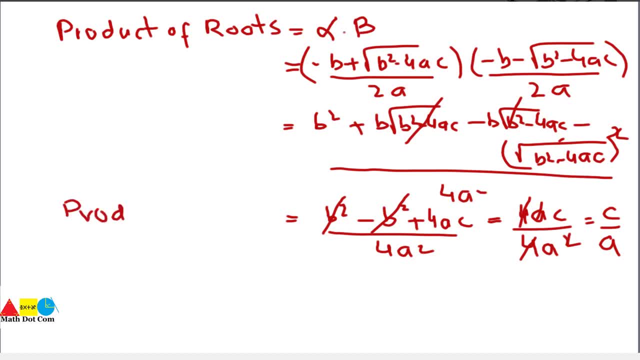 Hence the product of roots of quadratic equation r is equal to c by a. So we have got the two relations by using the relationship of sum of the roots and the product of the roots. So sum of the roots came out as sum of roots equals to, if we say the sum of roots is s.